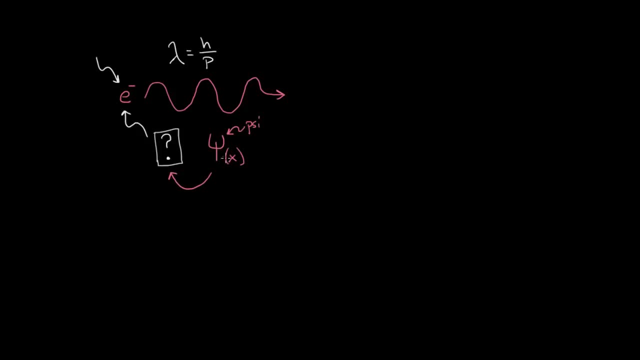 like: what does this wave function even mean? So we've got two problems: We want a mathematical description of the wave and we want to interpret. what does this wave even mean? Now, the person that gave us the mathematical description of this wave function was Erwin Schrödinger. So Schrödinger. 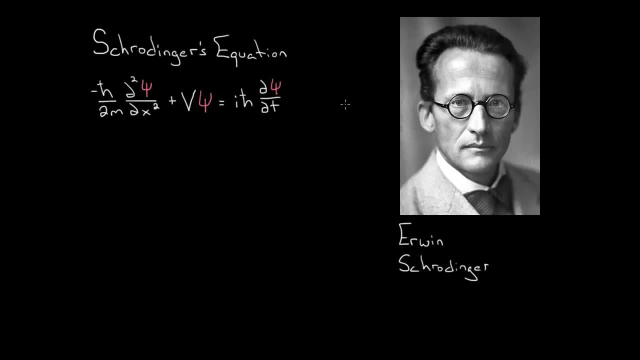 is this guy right here? Schrödinger is right here. He wrote down Schrödinger's equation and his name now is basically synonymous with quantum mechanics, because this is arguably the most important equation in all of quantum mechanics. 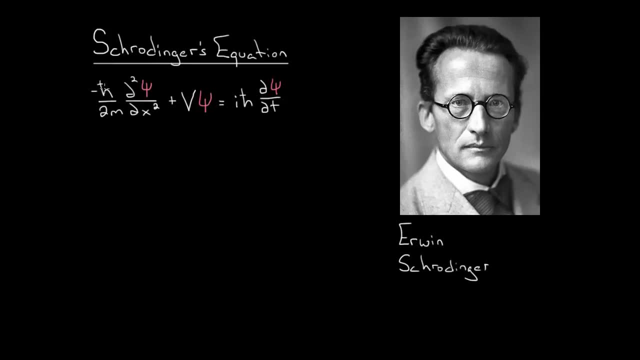 There's a bunch of partial derivatives in here and Planck's constants, But the important thing is that it's got the wave function in here. Now, if you've never seen partial derivatives or calculus, it's okay. All you need to know for our purposes today in this video is that 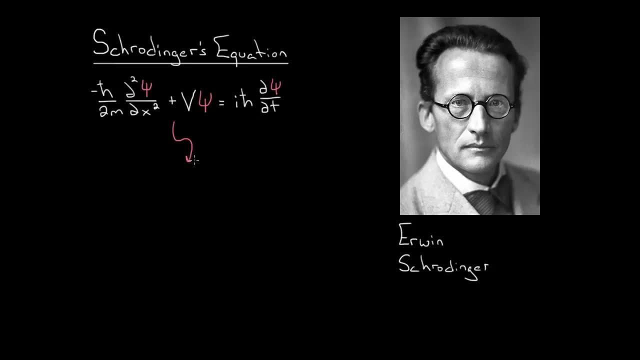 this equation is a way to crank out the mathematical wave function. What is this function? It's a function that gives us the shape of the wave as a function of x, And you could imagine plotting this on some graph. So once you solve for this psi as a function of x, you could plot: 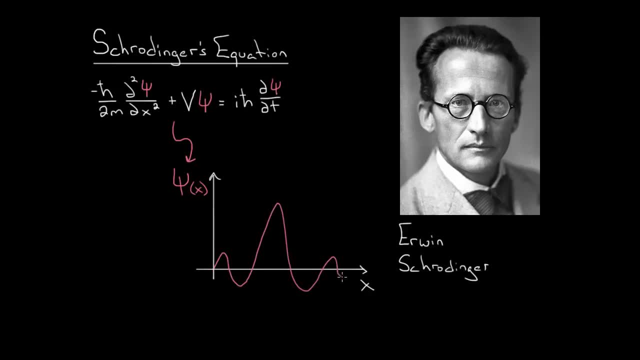 what this looks like. Maybe it looks something like this And, who knows, it could do all kinds of stuff. Maybe it looks like that, But Schrödinger's equation is the way you can get this wave function. So Schrödinger gave us a way to get the mathematical wave function. 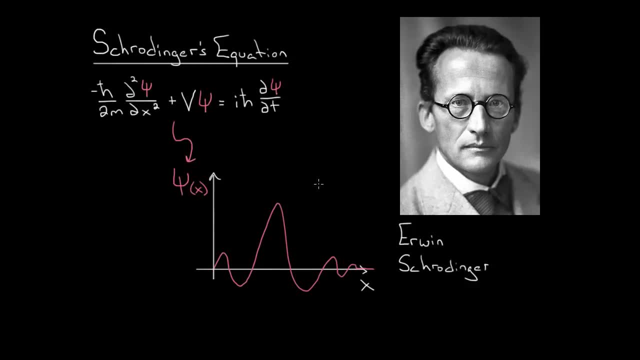 but we also wanted to interpret it. What does this even mean? To say that this wave function represents the electrons is still strange. What does that mean? Schrödinger tried to interpret it this way. He said: okay, maybe this electron really is like smudged out in space and its 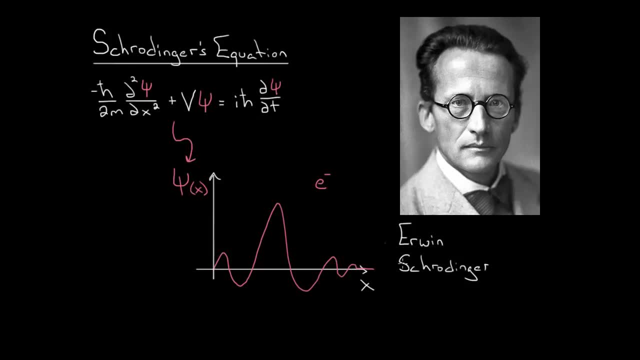 charge is kind of distributed in different places. Schrödinger wanted to interpret this wave function as charge density And I mean it's kind of a reasonable thing to do. The way you get a water wave is by having water spread out through space. So maybe the way you get 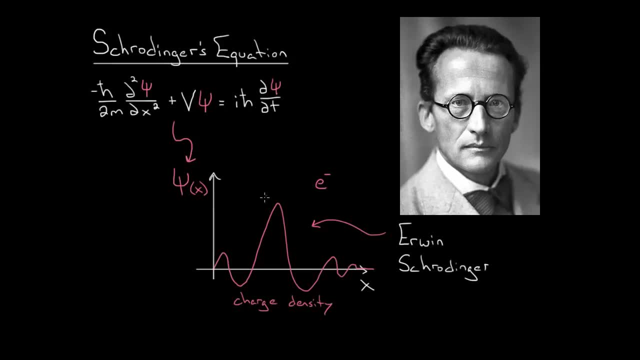 an electron wave is to have the charge of the electron spread out through space, But this description didn't work so well, which is kind of strange. Schrödinger invented this equation. He came up with this equation, but he couldn't even interpret. 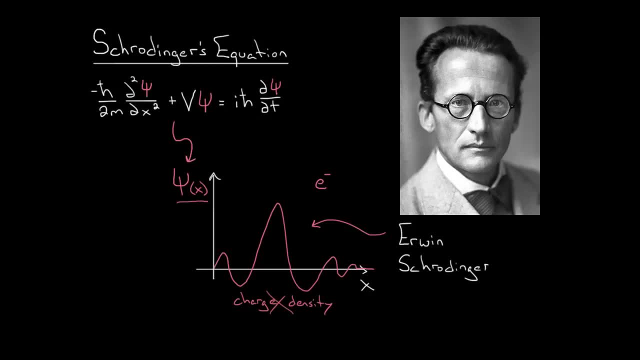 what he was describing correctly. It took someone else, It took a guy named Max Born to give us the interpretation we go with now for this wave function. Max Born said: nah, don't interpret it as the charge density. What you should do is interpret this psi as 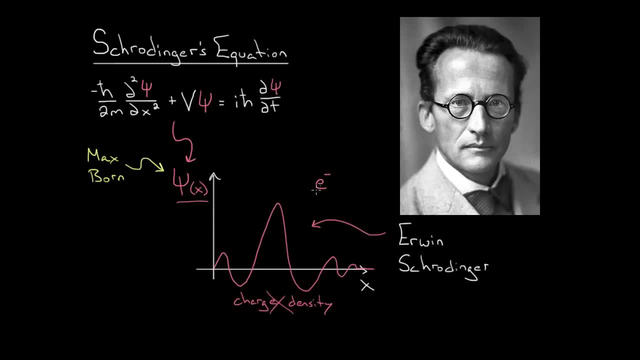 giving you a way to get the probability of finding the electron at a given point in space. So Max Born said this: if you find your psi, like he said, go ahead and use Schrödinger's equation. use it, get the psi. Once you have psi, what you do is you square this function. So take the. 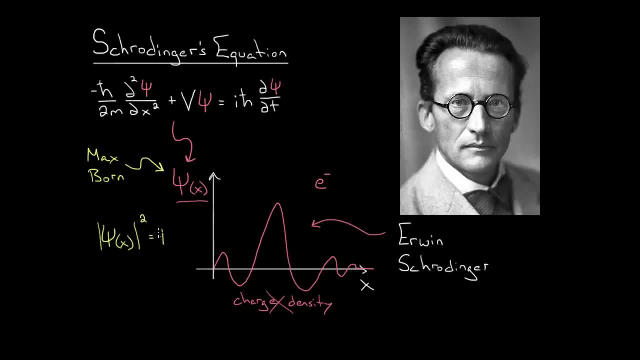 absolute value. square it, And what that's going to give you is the probability of finding the electron at a given point. Now, technically it's the probability density, but for our purposes you can pretty much just think about this as the probability of finding the electron at a given. 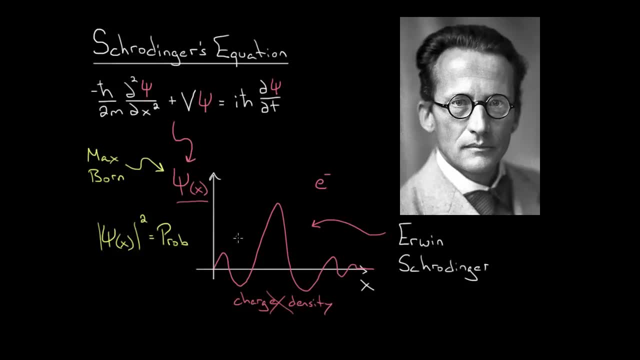 point. So if this was our wave function, in other words, Max Born would tell us that points where it's zero, these points right here, where the value is zero, there is a 0% chance you're going to find the electron there. Points where there's a large value of psi, be it positive or negative, there's. 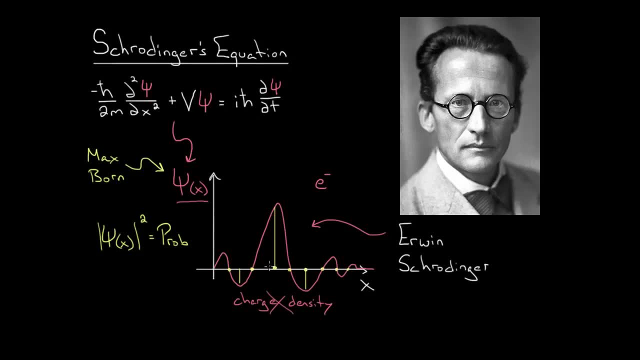 going to be a large probability of finding the electron at that point And we could say the odds point here are going to be largest for this value of x right here, because that's the point for which the wave function has the greatest magnitude. But you won't necessarily find the electron there. 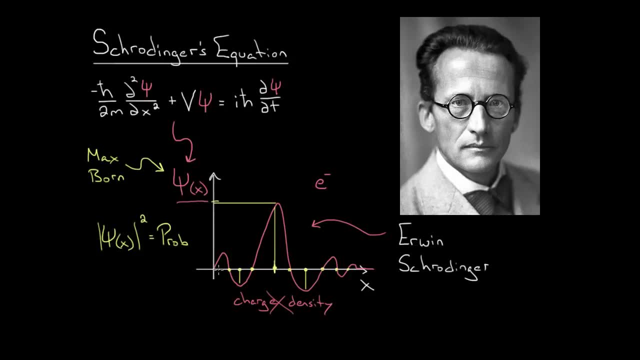 If you repeat this experiment over and over, you may find the electron here. once you may find it over here, you may find it there next time. You have to keep taking measurements and if you keep taking measurements you'll get this distribution, where you find a lot of them here, a lot of them. 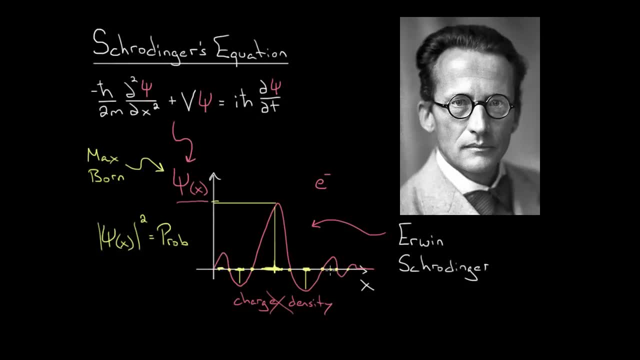 there, a lot of them here And a lot of them here. always where there's these peaks, you get more of them than you would have at other points, where the values were smaller. You build up a distribution that's represented by this wave function. So the wave function does not tell you where the electron is going to be, It just 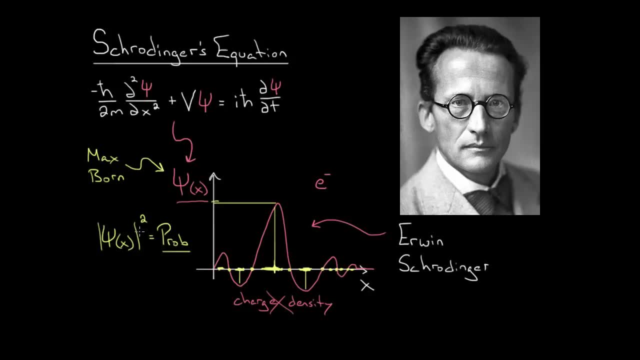 gives you the probability and technically, the square of it gives you the probability of finding the electron somewhere. So even at points down here where the wave function has a negative value- I mean you can't have a negative probability- You square that value. That gives you 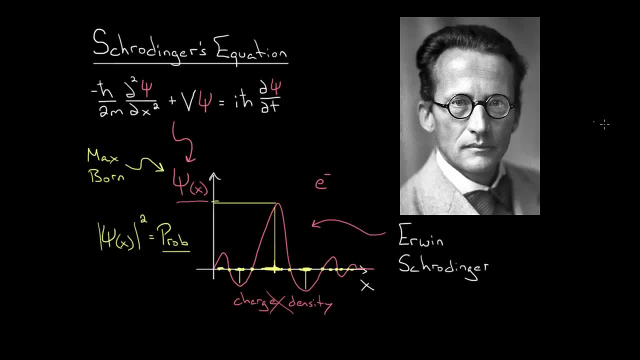 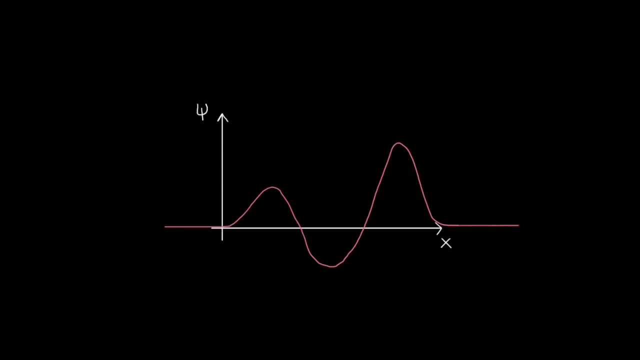 the probability of finding the electron in that region. So, in other words, let's get rid of all this. Let's say we solved some Schrodinger equation, or we were just handed a wave function and we were told it looks like this and we were asked: where are you most likely to find? 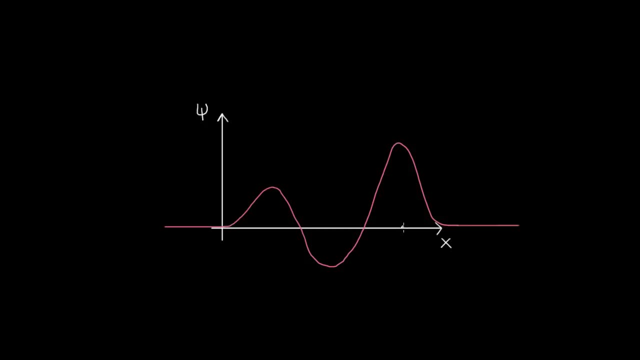 the electron Well, the value of the wave function is greatest at this point here, so you'd be most likely to find the electron in this region right here. You'd have no shot of finding it right there. You'd have pretty good odds of finding it right here or right here. 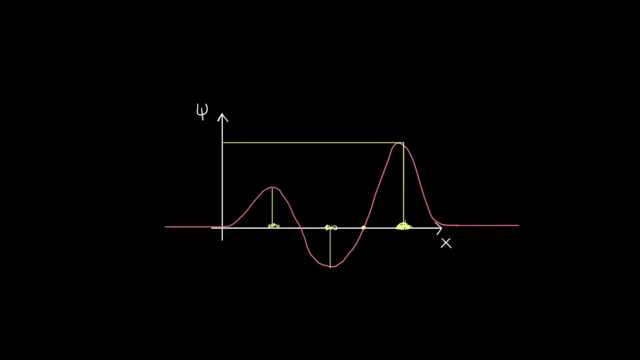 but you'd have the greatest chance of finding it in this region, and you'd have the greatest chance of finding it in this region right here, So you'd have to repeat this measurement many times. In quantum mechanics, one measurement doesn't verify that you've got the right wave function. 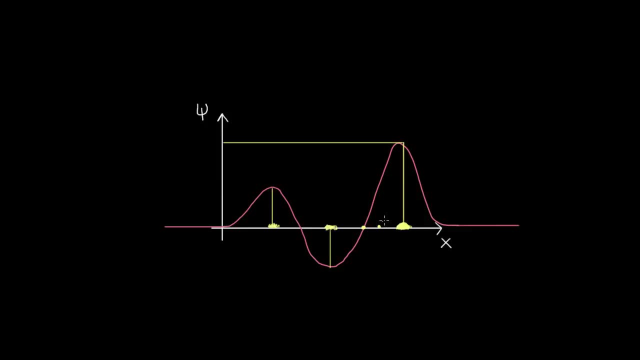 because if I do one experiment and measure one electron boop, I might find the electron right there. That doesn't really tell me anything. I have to repeat this over and over to make sure the relative frequency of where I'm finding electrons matches the wave function I'm using. 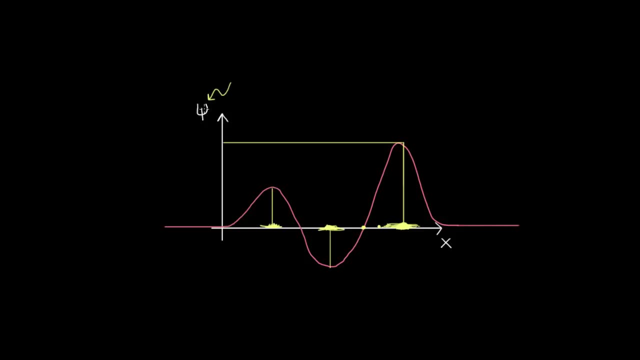 to model that electron system. So that's what the wave function is, That's what it can do for you, Although if I were you, I'd still be unsatisfied. I'd be like: wait a minute, Okay, that's fine, and 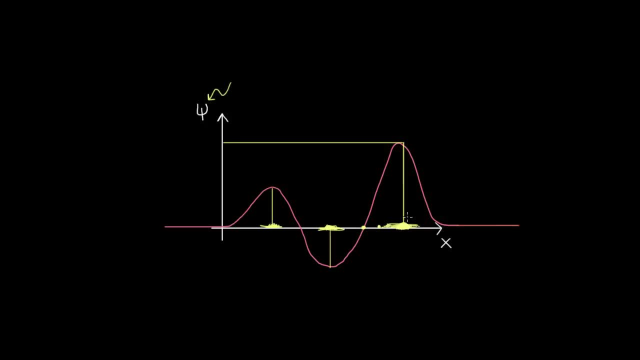 good Wave function can give us the probability or the probability density of finding the electron in a given region. but we haven't answered the question: what is waving here, And what exactly is this wave function? Is this a physical object, sort of like a water wave or even an electromagnetic 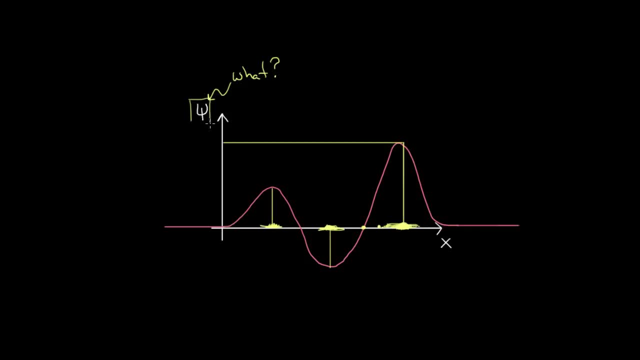 wave, Or is this just some mathematical trickery that we're using that has no physical interpretation other than giving us information about where the electron's going to be? And I've got good news and bad news. The bad news is that people still don't agree on how to interpret this wave function. 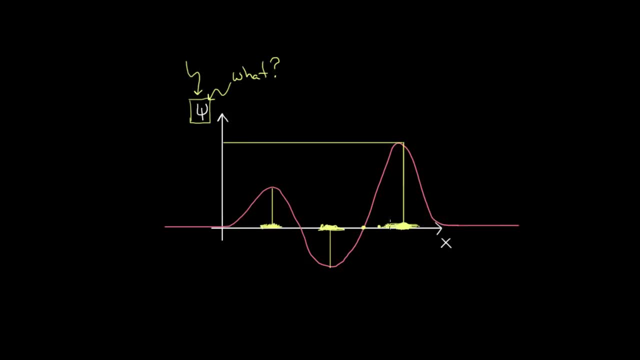 Yes, they know that the square of it gives you the probability of finding the electron in some region, but people differ on how they're supposed to interpret it past that point. For instance, is this wave function the wave function of a single electron, Or is this wave function really? 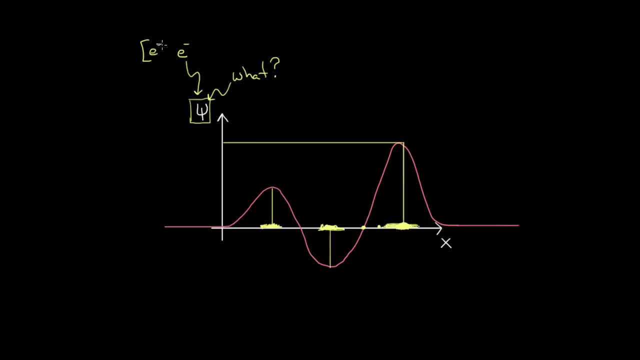 the wave function of a system, an ensemble of electrons, all similarly prepared, that you're going to do the experiment on. In other words, does it describe one electron or only describe a system of electrons? Does it not describe the electron at all, but only our measurement? 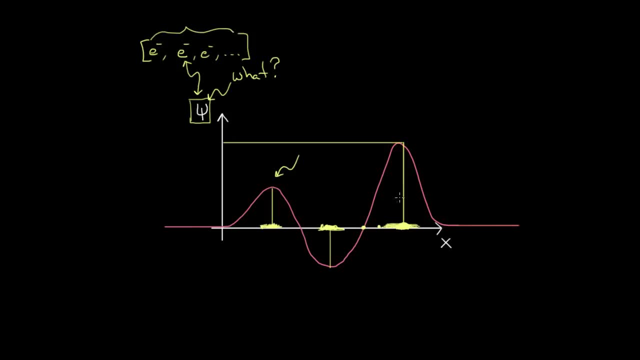 of the electron, And what happens to this wave function when you actually measure the electron? When you measure the electron, you find it somewhere, And at that moment there's no chance of finding it over here at all. So does the act of measuring the electron. 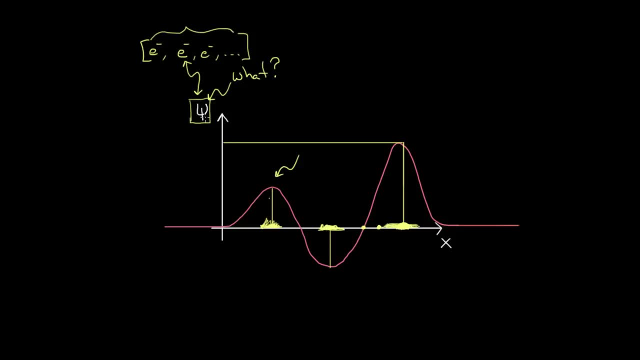 cause some catastrophic collapse in this wave function that's not described by Schrodinger's equation. These and many more questions are still debated and not completely understood. That's the bad news. The good news is that we don't really need to understand that to make 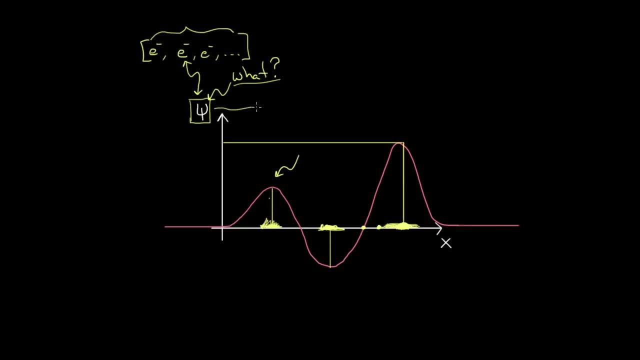 progress. Everyone knows how to use the wave function to get the probabilities of measurements. You can have your favorite interpretation, but luckily, pretty much regardless of how you interpret this wave function, as long as you're using the wave function, you're going to be able. 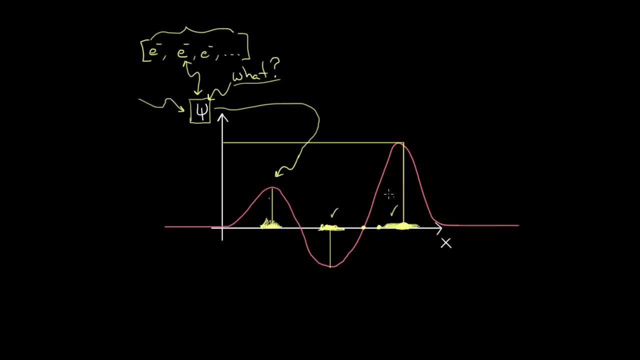 to get the probabilities of measurements. You can have your favorite interpretation, but luckily, pretty much regardless of how you interpret this wave function, as long as you're using the wave function you're going to be able to get the probabilities of measurements. You can continue making progress. 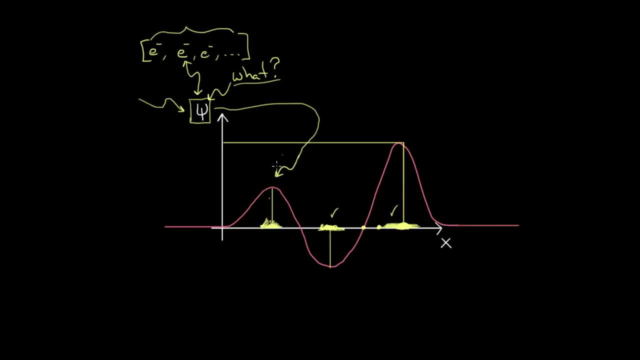 testing different models and correlating data to the measurements that people make in the lab. Now I'm not saying that interpretations of this wave function are not important. People have tried cracking this nut for over a hundred years and it's resisted. Maybe that's. 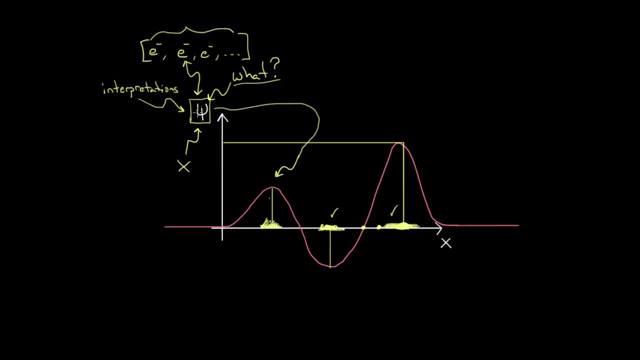 cause it's a waste of time, or maybe it's cause the difficulty of figuring this out is so great that whoever does it will go down in history as one of the great physicists of all time. It's hard to tell right now, but what's? 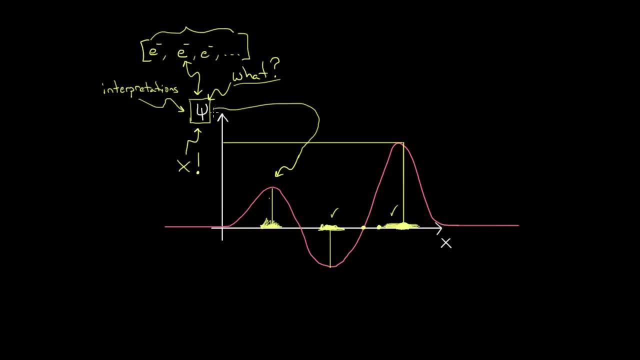 undebatable is that for about a hundred years now, we've been able to make progress with quantum mechanics, even though we differ on how exactly to interpret what this wave function really represents. So recapping the wave function gives you the probability of finding a particle. 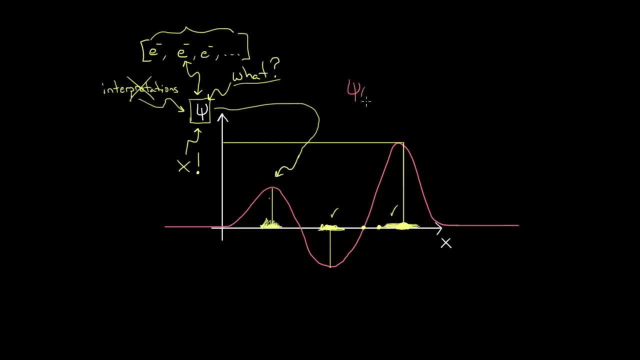 in that region of space. Specifically, the square of the wave function gives you the probability density of finding a particle at that point in space. This almost everyone is a agreed upon. Whether the wave function has deeper implications besides this, people differ, but that. 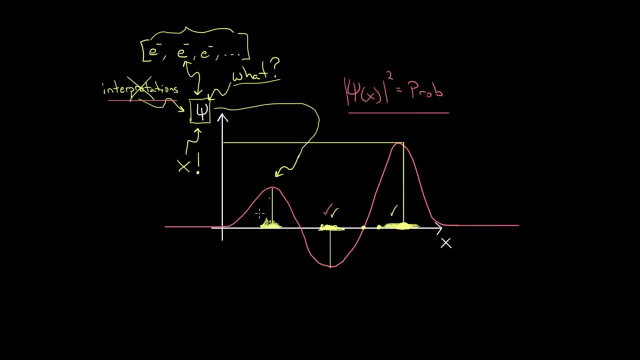 hasn't yet stopped us from applying quantum mechanics correctly in a variety of different scenarios.